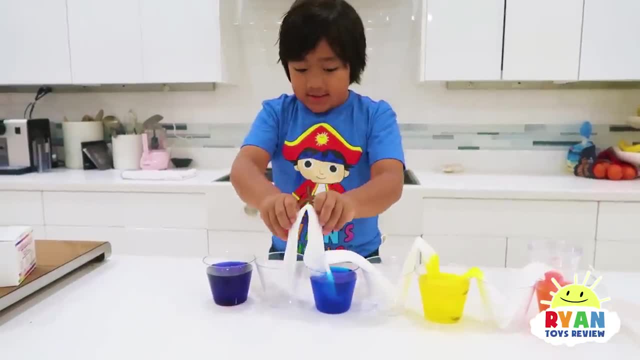 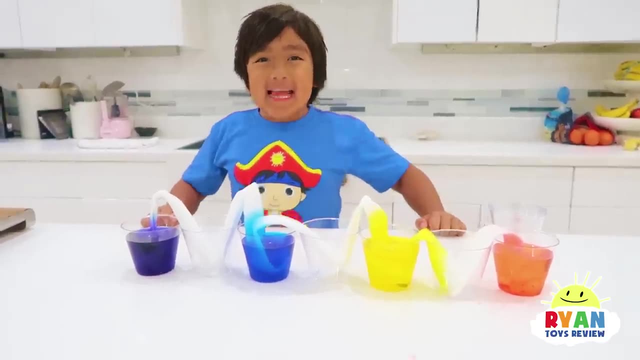 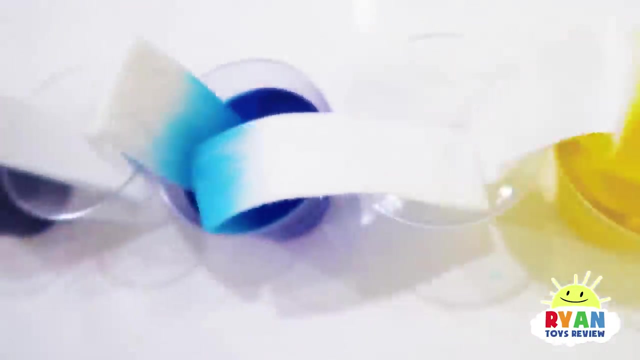 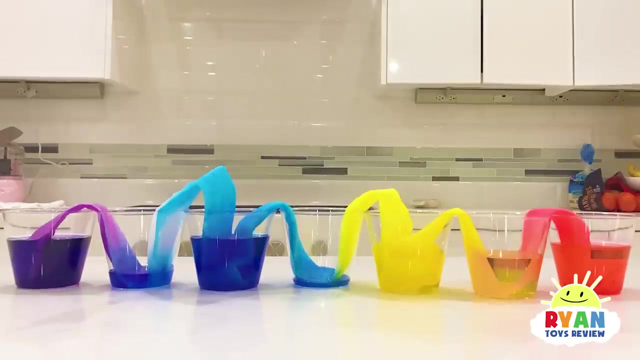 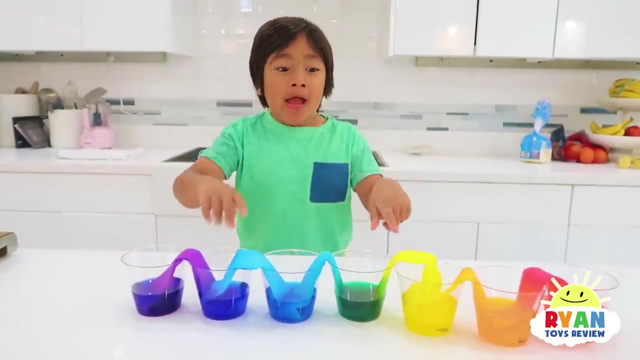 And this And this And last one Like this. Now we just have to wait and see what happens. Look, the water's already traveling up the paper towels. Guys, it's the next day and look what happened. The water went up the paper towels and went down and mixed the colors together. 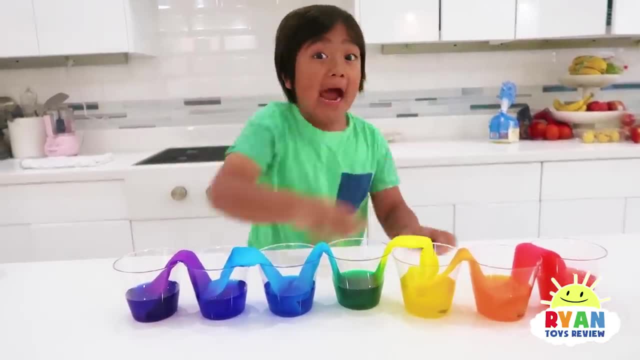 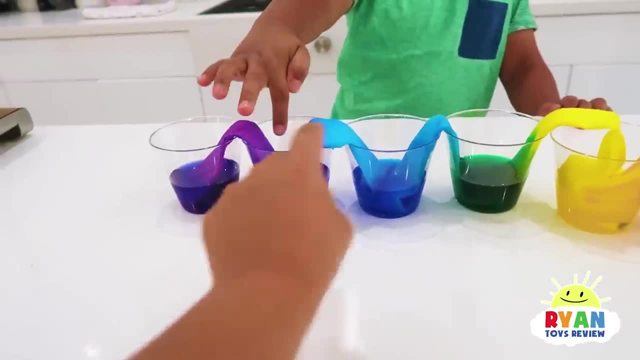 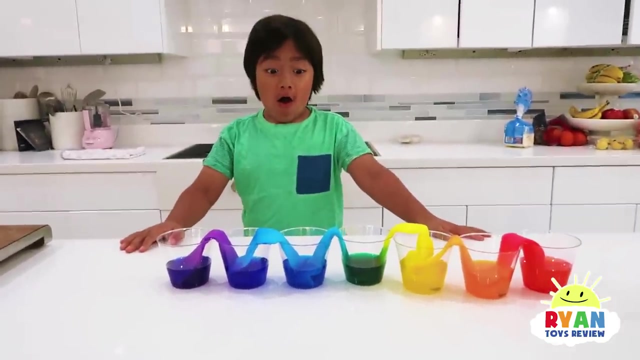 Look, and now, the cups that were empty now has water. See what happened, Ryan. The water travels up and then over. And then this cup: the water travels up and then also over, right? So how did the water travel up the paper towel? 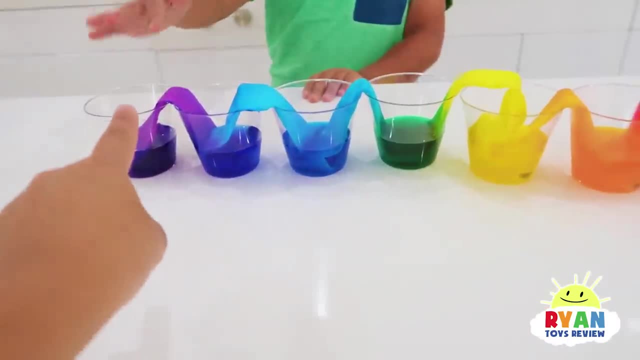 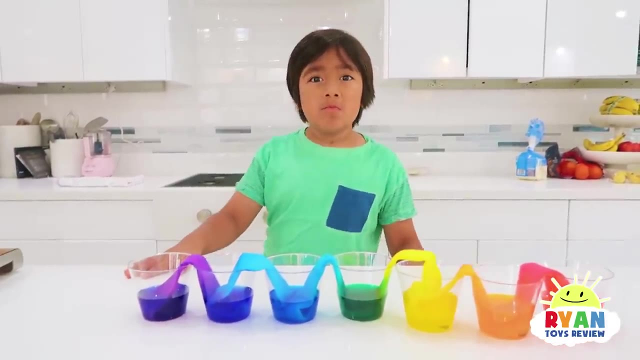 Here's how it happens: The water color travels up the paper towel by this thing called capillary action. So do you remember how plants? where does the plants get the water from? Like underground? Yeah, underground, That's right from the roots. 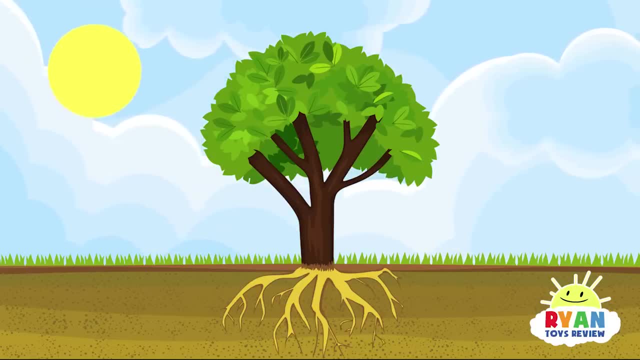 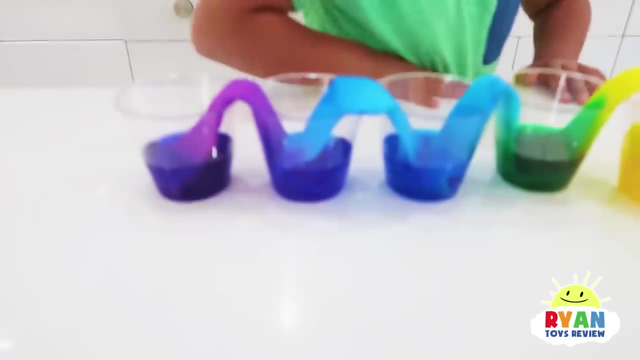 So the plants get water from the roots but it has to travel up the plants So, against gravity. So it takes the water from the ground and travel it up, just like how the paper towel takes the water from the bottom and it travels up. 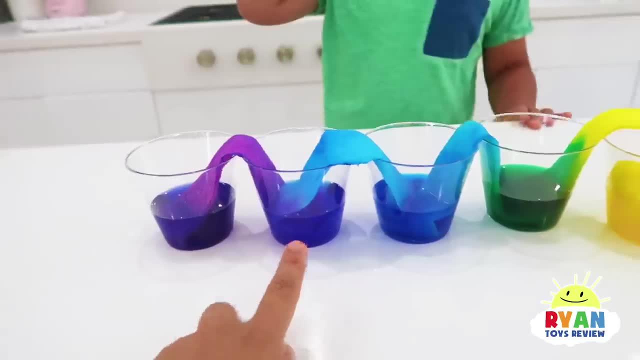 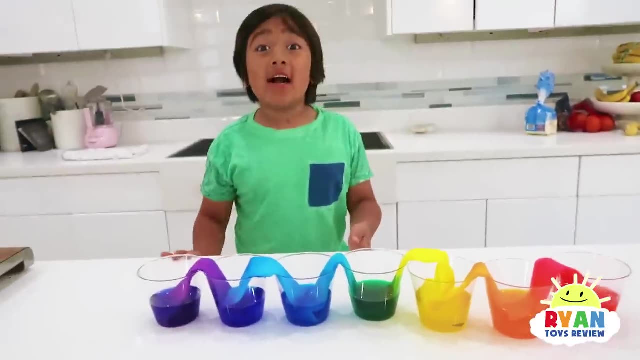 Now you see how the empty cup changes colors. Yeah, Okay. so here you have blue with yellow. When you mix blue and yellow together, what did you get? I got green, That's right. And here you have yellow mixed with red. 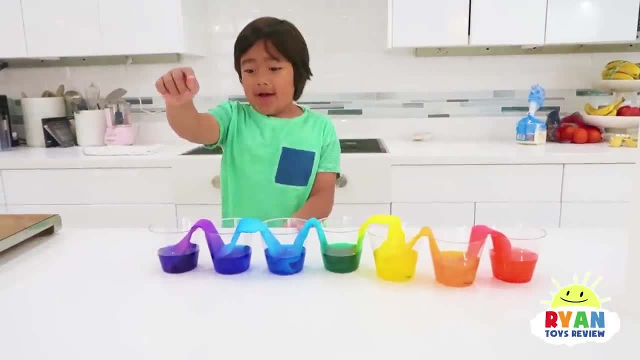 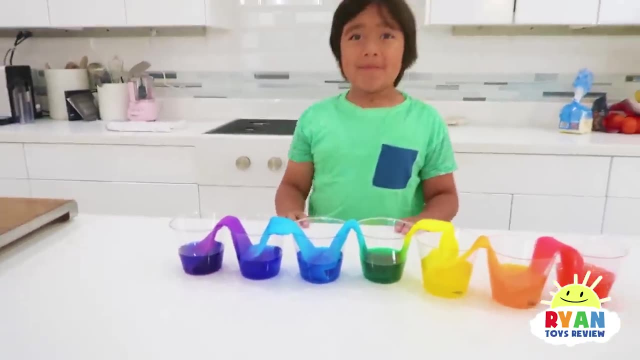 What do you get? Orange, Orange, yeah. And blue and purple is like a galaxy color. That's right, Yeah. so what happens when you mix it together? That's so cool, right Yeah? Now let's take out the paper towels and see what it looks like. 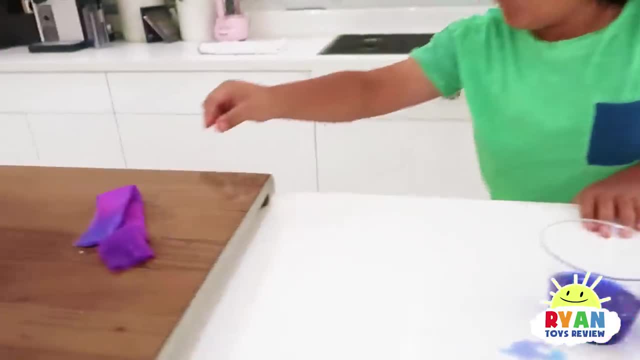 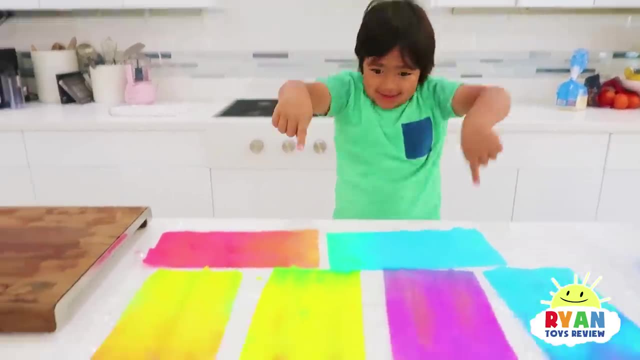 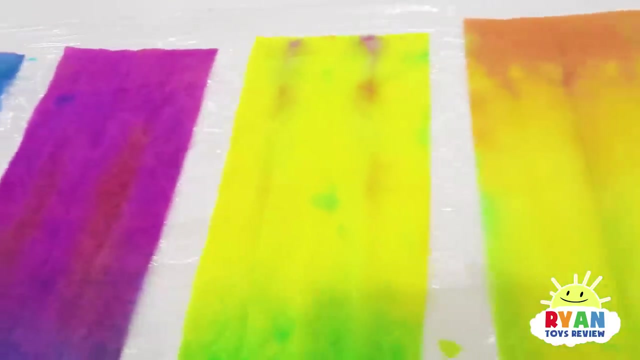 Cool And blue. Here's what it looks like when we take out the paper towels. Look at all the colors. It looks like a tie-dye t-shirt. Yeah, Wow, you guys see. Yeah, It's really really cool.